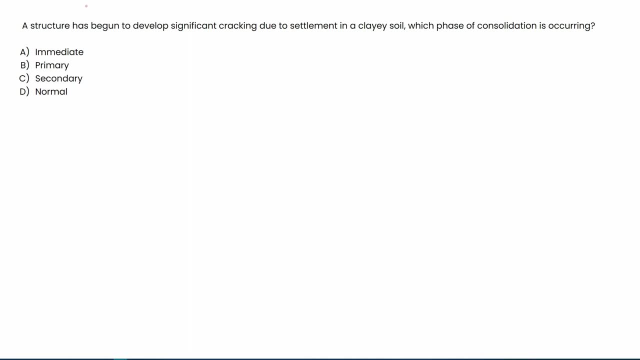 We're going to be in soil mechanics and soil consolidation, And so here's what the question says. A structure has begun to develop significant cracking due to the settlement in a clayey soil. Which phase of consolidation is occurring? It gives us our four options. immediate, primary. 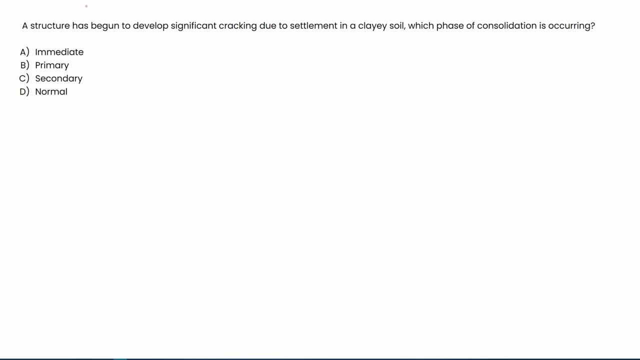 secondary and normal, And so the first thing that we need to do is find some reading material. And, granted, this doesn't have a lot of information applicable to this problem, but it does have some good information that might help with the background of the problem. 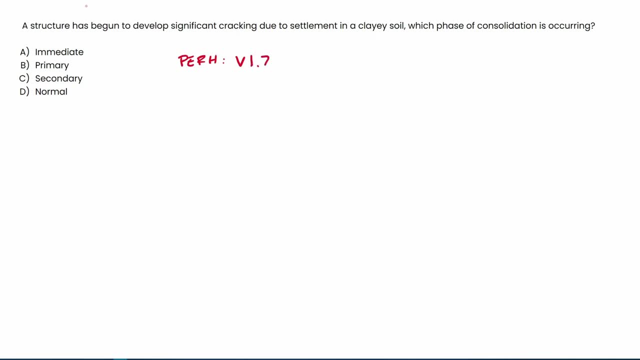 So we're going to be looking in the PE reference handbook version 1.2.. That's the latest and greatest at the point of this recording. We're going to be looking in chapter three and that is the geotech section in the manual. 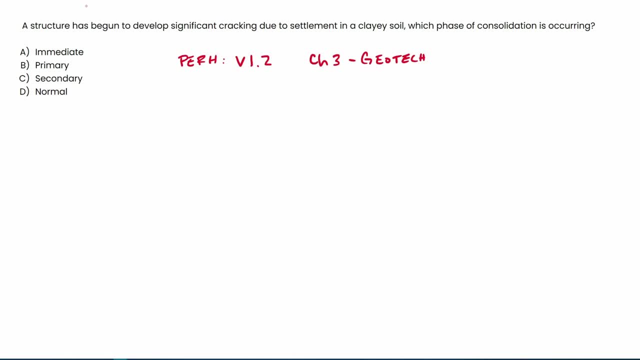 And so there's actually no real answer. Like I said earlier, the answer isn't in the manual. There's just really good information in chapter three that might be applicable to this. You can kind of do some digging and do some research there. But I guess if I'm going to go down the 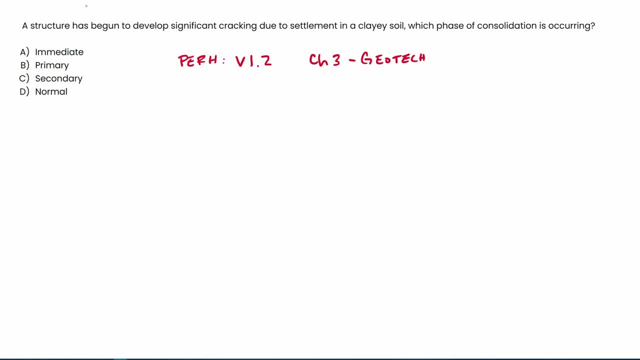 list here: immediate settlement. that's going to be almost like an elastic settling. That's sometimes what they'll call it, And it's actually immediately after a structure is constructed And you'll see it usually in some kind of sand material, that type of thing, And in our 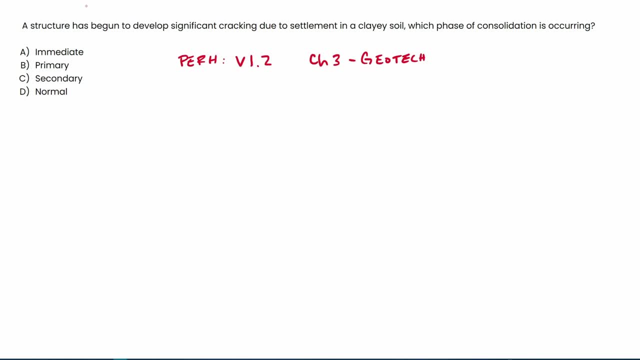 problem statement. they actually give us a huge hint: clay clayey soil. So it's a clay type soil. So we know immediate settlement is probably not going to be the answer to this one. It's almost like one of those like which are the best answers types of thing. So here's B, let's see. 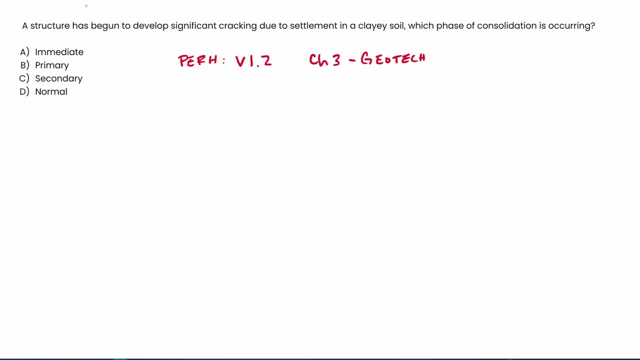 primary. The primary actually occurs gradually in clay and it's due to the water leaving the void spaces. So kind of think about it that way. And then C secondary, that actually occurs over a longer period of time. It's a slower rate. 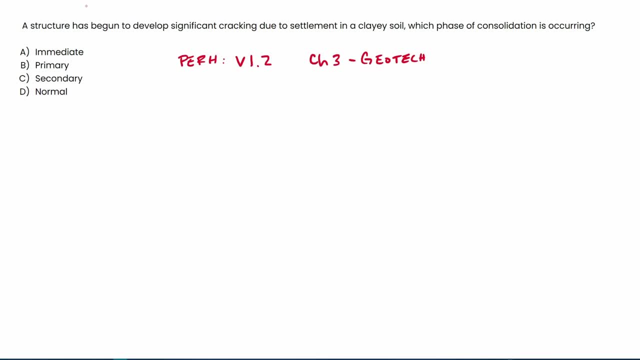 And it actually happened to clay soils as well, And it's really just the readjustment of the soil particles, finding their finding, finding their final resting place- tongue twister there But- and it's way less magnitude than primary, I mean you can imagine- just little tiny soil particles.